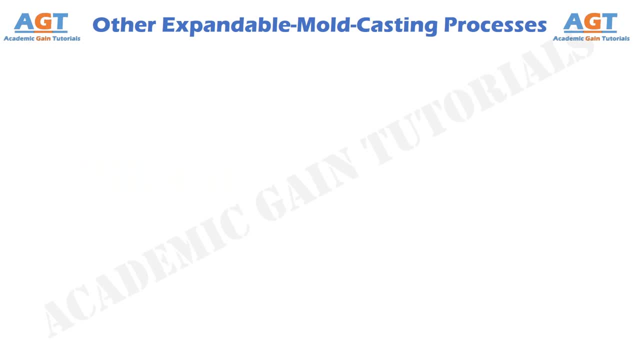 Except sand casting, there are other casting processes that have been developed to meet special needs. The difference between these methods are in The composition of the mold material, Or the manner in which the mold is casted, Or in the way the pattern is made. In investment casting, a pattern made of wax is coated with a refractory material to make the mold, after which wax is melted away prior to pouring the molten metal. 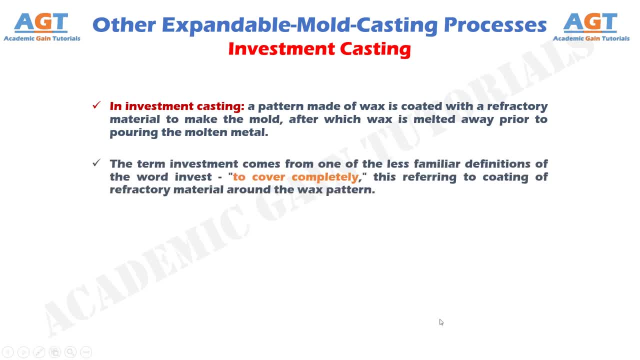 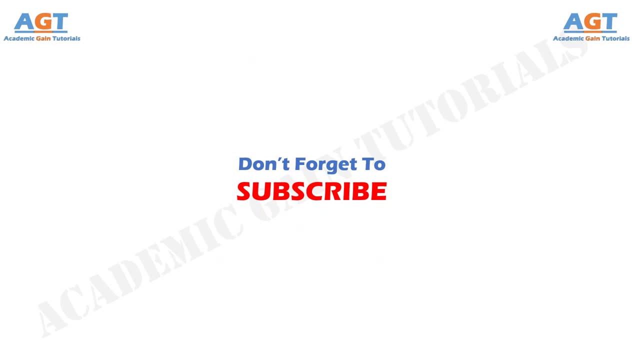 It is a precision casting process as it is capable of making castings. It is a precision casting process as it is capable of making castings. It is a precision casting process as it is capable of making castings. Thanks for watching.